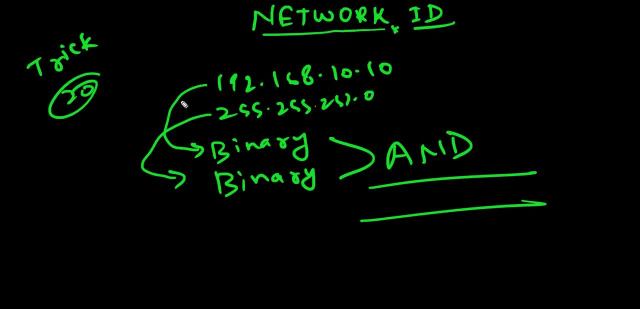 that will. It will be your network ID, Fine, But it is a lengthy process. It will take approximately one to two minutes to calculate network ID, Right? So what is the trick to calculate network ID within 20 to 30 seconds? Let me show you. Let me show you today. Okay, Let me remove. 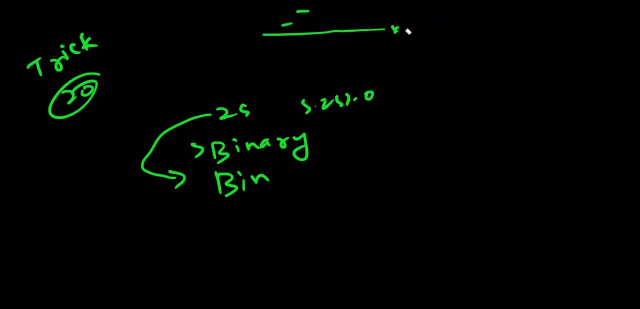 it. Let me show you. Just suppose I have one IP address, 192.168.10.10.. Subnet mask: 255.168.10.. Suppose I have one IP address, 192.168.10.10.10.. Suppose 95 and slash 25.. Right, If someone. 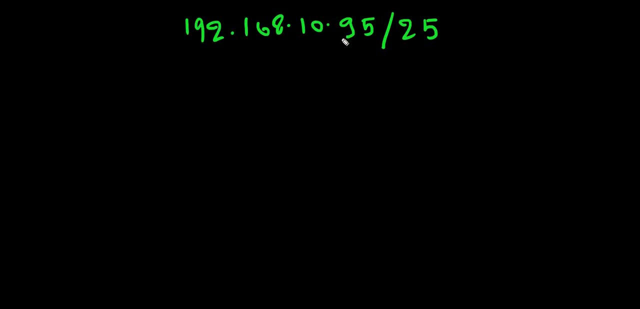 will ask you this IP address belongs to which network, Right? Or a person can ask you find the network ID of this IP address, Right? So The interviewer can ask a question in different way, Right? The interviewer can ask you: please tell me this IP address belongs to which network, Or they can ask you to find network ID of. 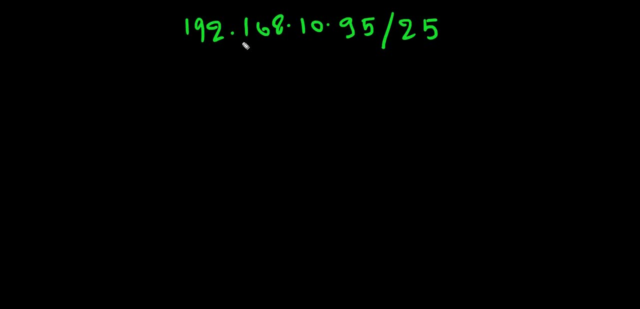 this network Right. Or they can ask you to find first valid IP address of this IP, of this IP address Right. First valid IP address. Last valid IP address: Broadcast ID, Network ID Right. So today I am going to show you how to calculate network ID with trick Right. 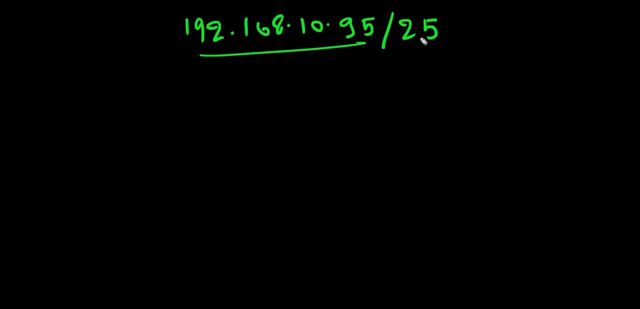 So what you need to do over here is you need to write subnet mask of slash 25.. As you know, subnet mask will be 255.255.255.128.. Right, Don't need to focus over here and don't need to write these. all things You can. you can write subnet mask of fourth octet, Right. 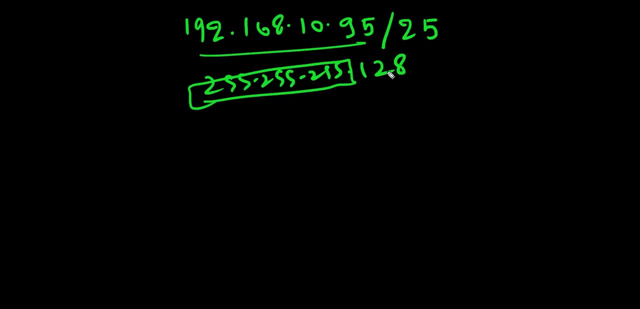 Because you know the last one is present in fourth octet, Right. So you can write the subnet mask of fourth octet, Right, So you don't need to write this complete information. Just try the subnet mask of last octet, Last octet, Subnet mask of that octet where last. 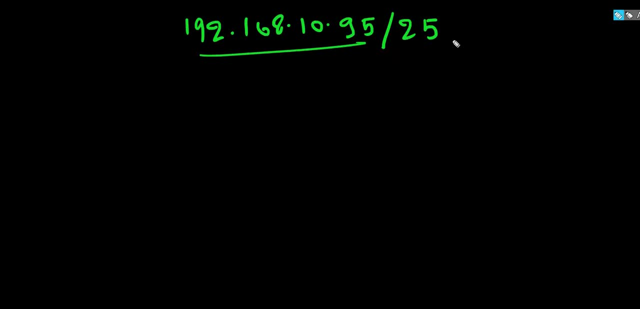 one is present. So in my case I am using slash 25.. That means last one is present in fourth octet, Right? Last one is present in fourth octet. So let me write the subnet mask of fourth octet. Subnet mask of fourth octet is 128.. 128. Right, Just you need to write. 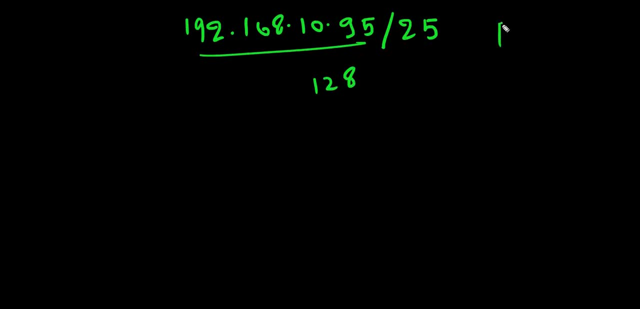 subnet mask of last octet 129.. Right, Find blocks. Right, So you need to find blocks. Block size: Block size will be 256 minus 128. Then you will get 128.. Right, That means your first network will be 10.0.. Your second network will be 10.128.. So this network will 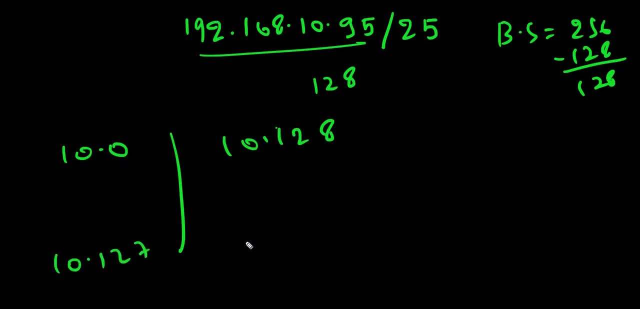 end here 10.127.. And this network will end over here 10.255.. Right, So this IP address belongs to which network? This network or this network? Right, So, in this network. So what is the network ID for this IP address? 10.10.. 10.0.. Sorry, 10.0.. Let me discuss. 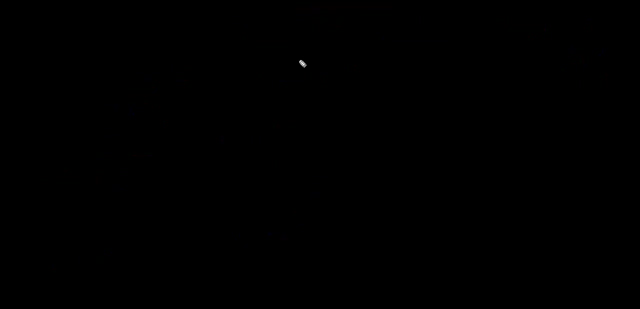 one more question, Right? If you are thinking, sir, it's taking approximately 1 to 2 minutes, Just wait here. Just wait, Right? You can calculate network ID of any IP address within 20 seconds. It's my promise. Just wait. See, I have one another IP address, The same IP. 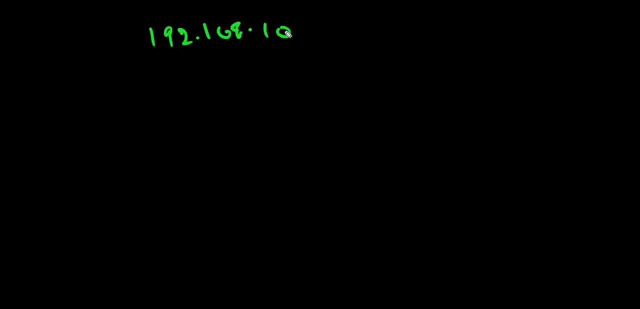 address: 192.168.10.. Right, So this IP address is 192.168.10.. Right, So this IP address is 192.168.10.. close to 192.168.10.. That's the one IP address for your IP address, How many? 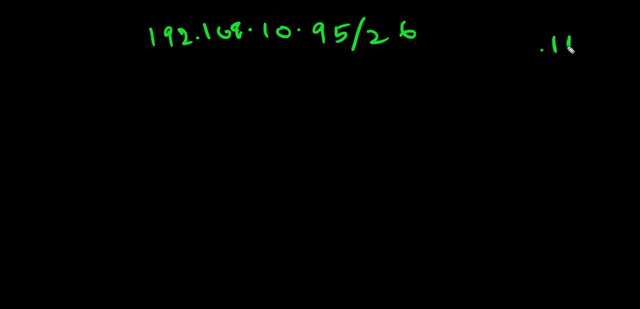 IP addresses. you have 205, or only 205?? No, 188.. Can you calculate that? No, No, ruthen values are different. Allholders belong to this network. Anyway, we need to deal with the end of IP addresses, here or in deltas. Well, let me tell you guys, Obviously you will just locate. 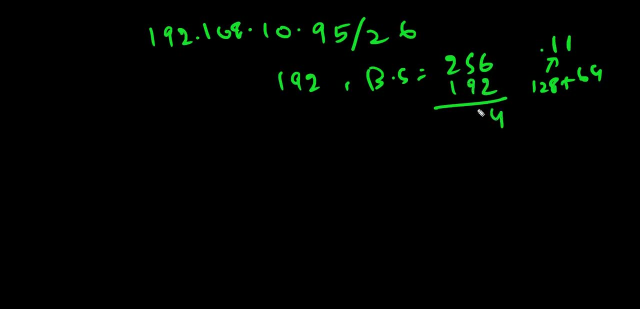 this network and here 6, so 64. you are getting 64, right, you don't need to do anything, just divide your, your value, which present in fourth octet, by 64, by block size, right? so value in fourth octet is 95. let me divide by 64, right, so 164. you will get 1 and 9 minus 1 over here, and we have 9, so we have. 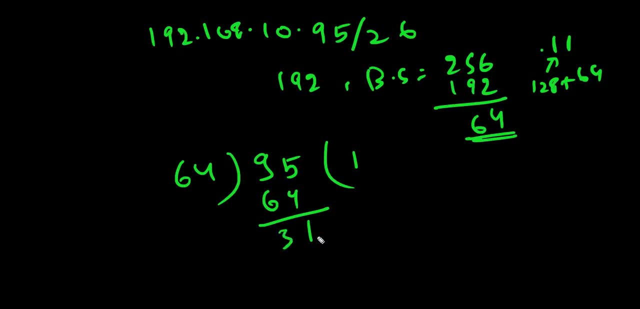 2 minus 6, so 3, 31. i am getting 31 over here right now. subtract this 31 to 95, right? so 90, 95 minus 31. what you will get? you will get 4, 6, 64. that means network id of this particular ip address. 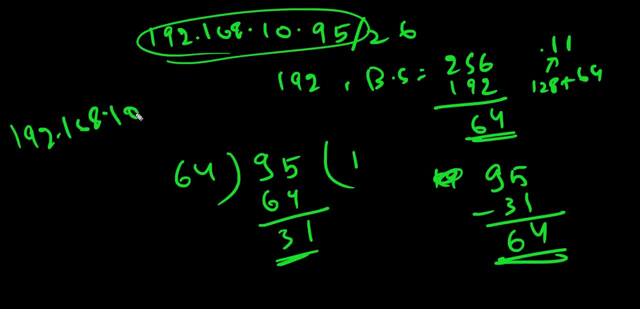 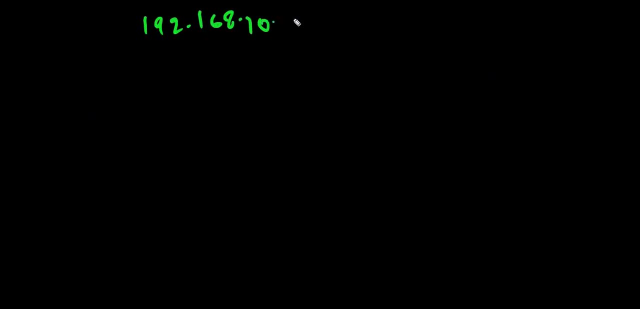 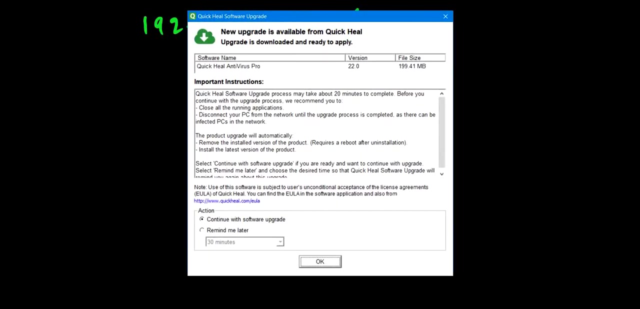 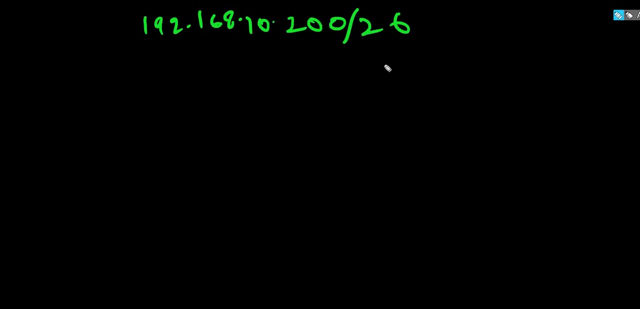 is 192.168.10.64. 192.168.10.64, right. just suppose i am using 192.168.10.10.10.64 200, right, and slash 26, slash 26, okay. so what will be the subnet mask of last last octet? again 192. so 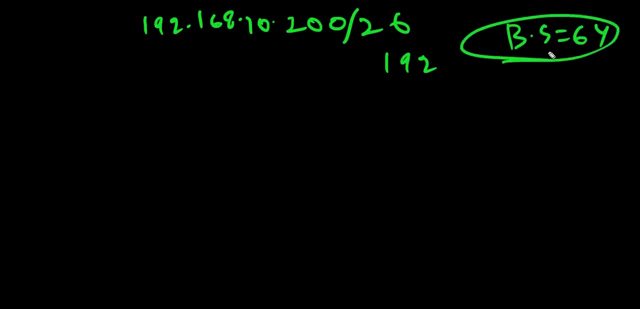 what will be the block size? again, block size will be 64 am i right now divide 200 by 64, so 64 and 200 right. 3, 4, 3 is a 12 and 6, 3 is a 18, 190 right. subtract it. so 10 minus 2 is 8 right. 9 minus n is 0. 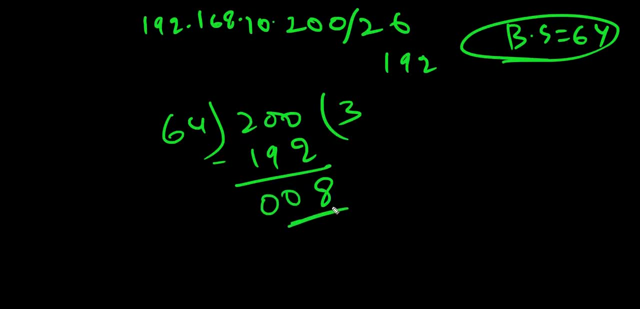 0, right, so i am getting 8. so you now subtract this 8 from 200, 200 minus 8, right, you will get 192. that means network id of this particular ip address is 192.168.10.64 dot. 10.192. right, this is the network id. this is ip address. right, this is ip address, right? don't say: 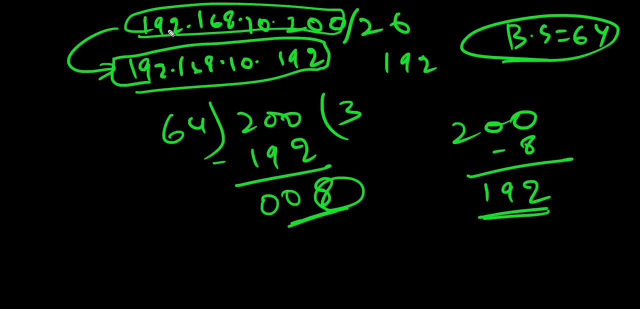 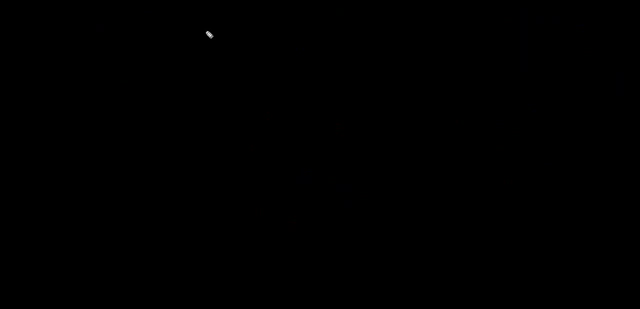 network id of this particular ip address is 192.168.10.0. i am using slash 26 over here, guys. network id will be 192.168.10.192. okay, let me. let me do one more question over here. same question: 192.168.10.10.200, and now i am using slash 27. so what will be the submit mask? 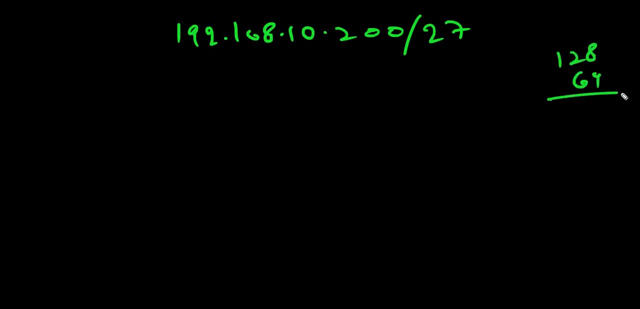 128 plus 64 is 192 plus 32, am i right? so 4 2, 2, some subnet mask of last octet will be 2 to 4. so what will be the block size? block size will be 256 minus 2 to 4 subtracted, so 2 and 3, 32 now i. 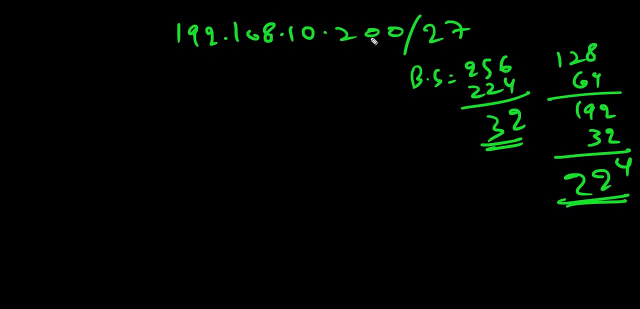 am getting block size 32 right now. let me divide 200 with 32, so 32 and 200 right six time i think. six time. so six, two zero twelve two, one eighteen and one nineteen right 192. again i am getting 192. so what value i will get over here? i will get eight. 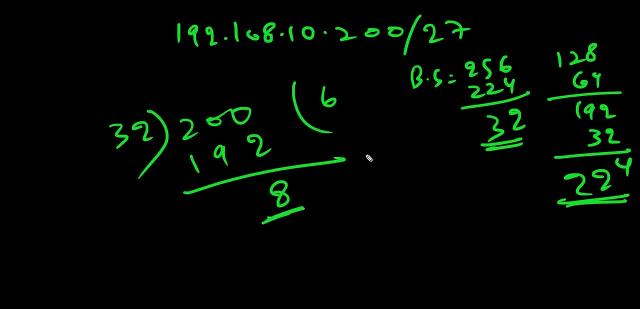 nine zero, zero. so i am getting eight. yes, subtract, subtract it 200, 100 minus eight, 192. again you are getting 192 network id, right. so this ip address is belongs to which network network: 192.168.192.168.10.10.192- 192. am i right? 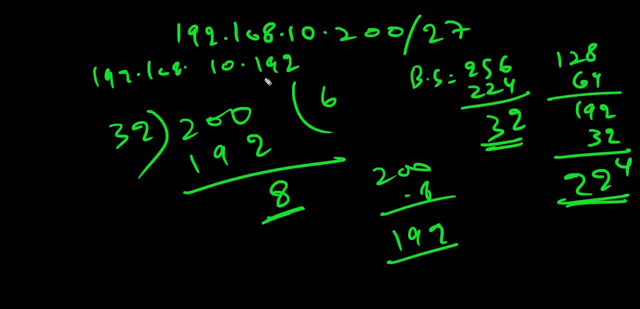 so in the same way you can calculate the network id of any ip address, of any ip address, right? you need to find block size. only after that, divide the value which present in last octet by your block size. okay, then, if you will get some value over here, if you will get some value over here, you. 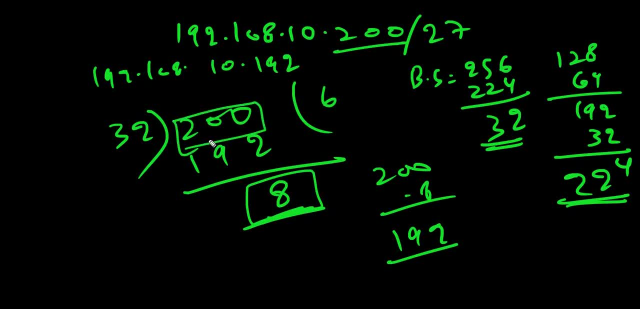 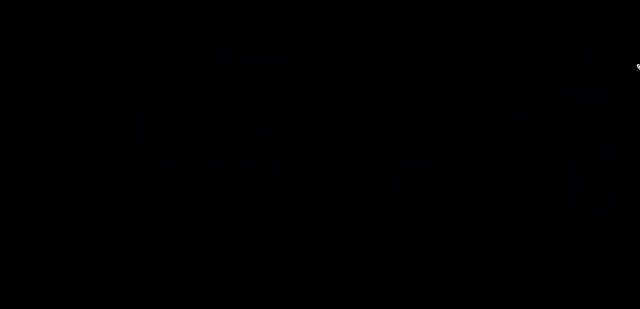 need to subtract that value from the value which present in last octet, then you will get network id. then you will get network id. fine, so thank you if you like this video, if you like this trick, please like the video. if you haven't subscribed my channel, subscribe this channel to get update.